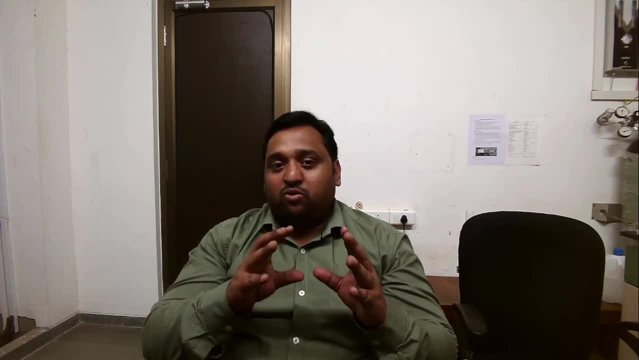 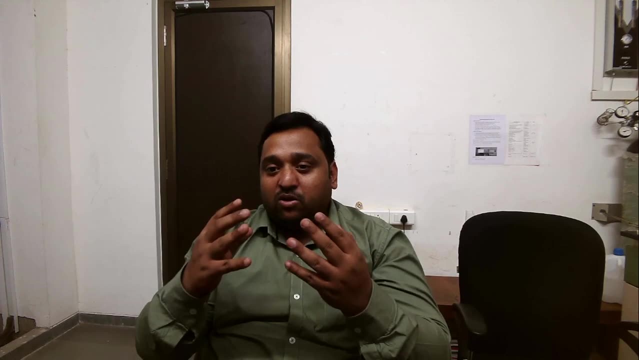 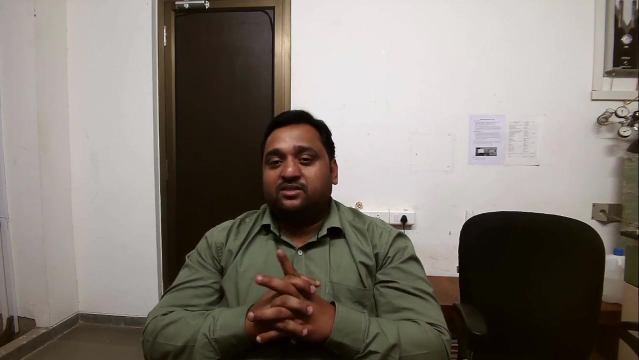 in our control. if I say amount of A has been increased to the reactor, this much amount, stoichiometrically, amount of B also should be increased to an extent of what A. okay, That is what the ratio control does, the job of this, matching the proportions of amount. 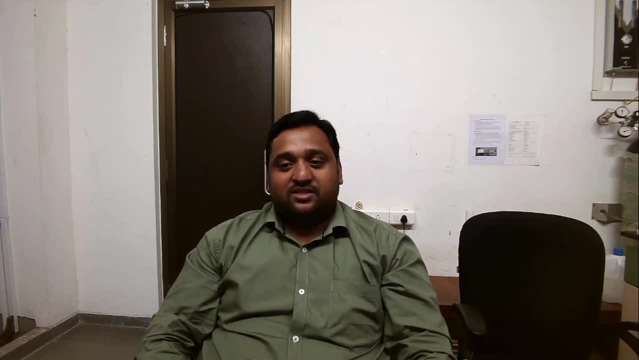 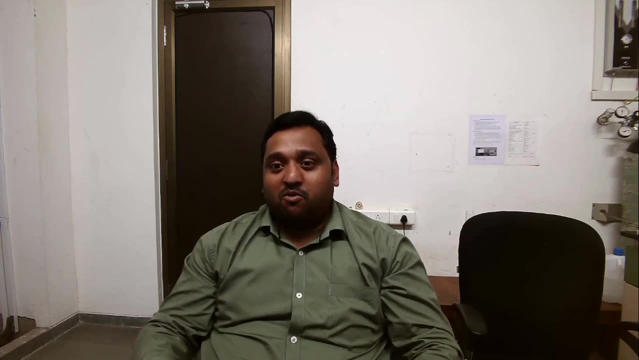 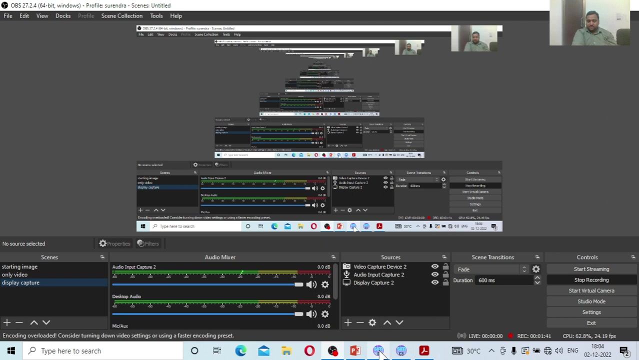 of A to the amount of B. okay, Today we are going to discuss ratio controller. So what is ratio controller? What is ratio controller? And you can imagine that it is a kind of- you know, feed forward kind of controlling. Let me explain you to the once you go to the simulator model. okay, 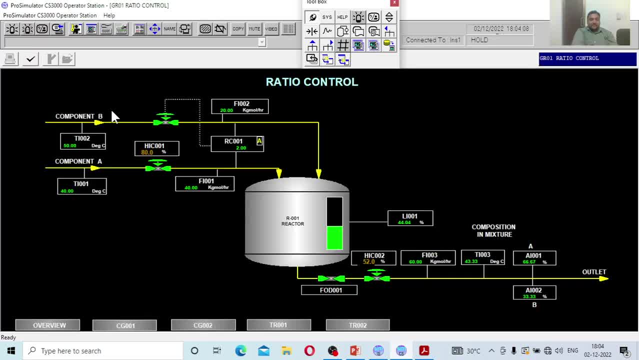 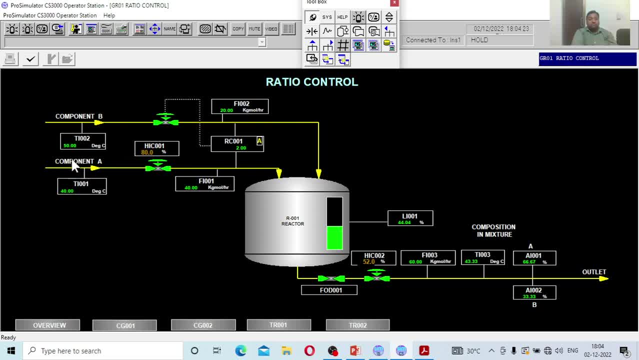 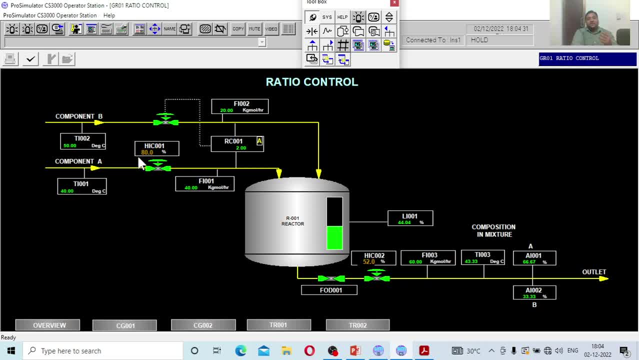 If A comes to this vessel and let us say A and B are getting reacted, the B also should come according to what A has increased into the reactor. Imagine saying this is the stream line of A which is coming into the reactor and stream line of B is connected to a ratio controller. 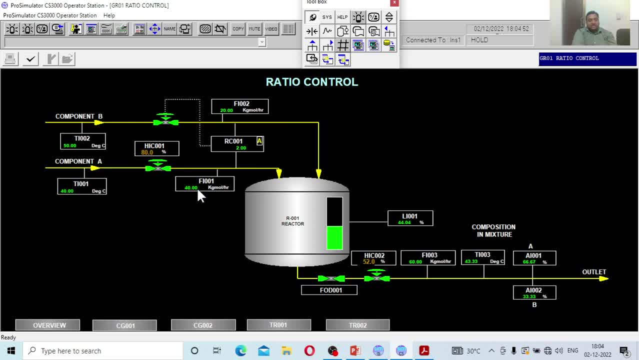 What it does. Let us example: if A is 40 kilogram mole per hour, then what? and the ratio B is maybe by 2 of A. that means 20 kilogram per mole of hour should go in accordingly. So presently you can see the operation. A and B are going into the reactor. A is 40, accordingly. 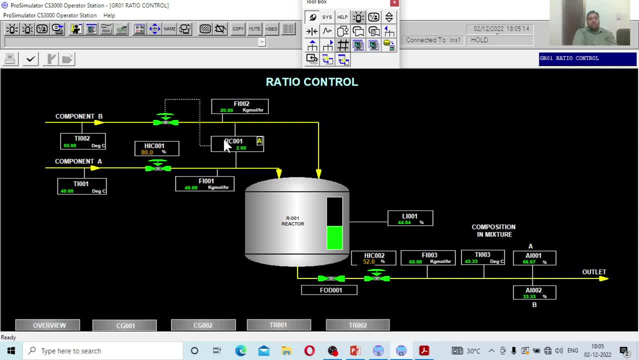 it will measure the flow rate of A and it will cross check with the stoichiometry and it will accordingly. the amount of P is going into the reactor Currently 40 kilogram per hour of A and accordingly half of the A, that is, B, is going into this. 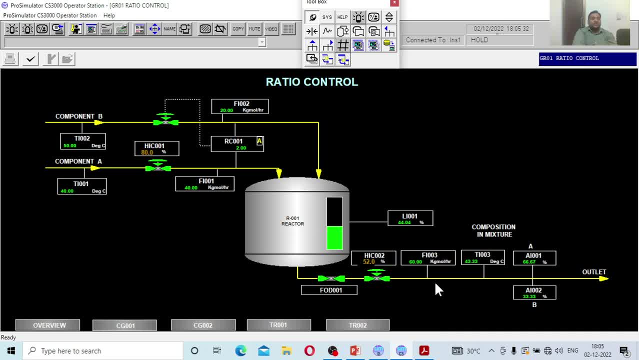 reactor and both are trying to exit the reactor and you can see the indicators. this is the indicators. this is temperature of A. temperature of B, the hand indicating control here. finally, total more total is 60, which is 40 plus 20, equal to 60. that exit temperature is. 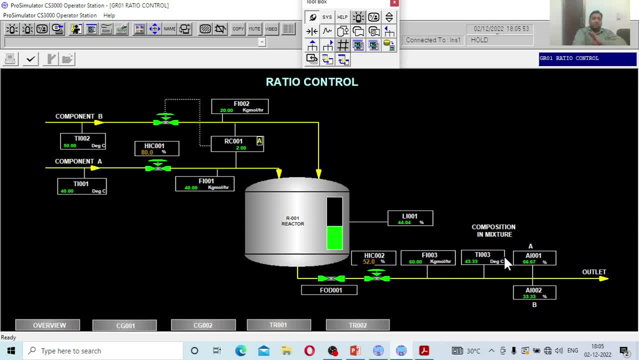 of the both the components is 43.83. this is just a quite not kind of reaction that is happening. it is simple kind of stoichiometric mixing that are going inside this particular vessel. The name is reactor but is no as such reaction that is happening. imagine that, say the exit. 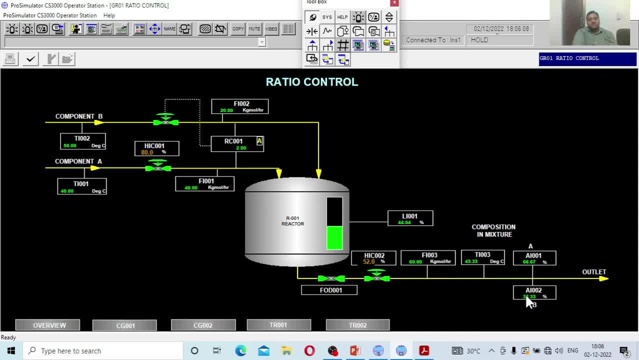 of this tank is: A is 66.67 percentage and B is 33.33 percentage. according to this amounts, 20 by 60 is called 33 and 40 by 60, I mean, is called 66. So it is a kind of stoichiometric amount. 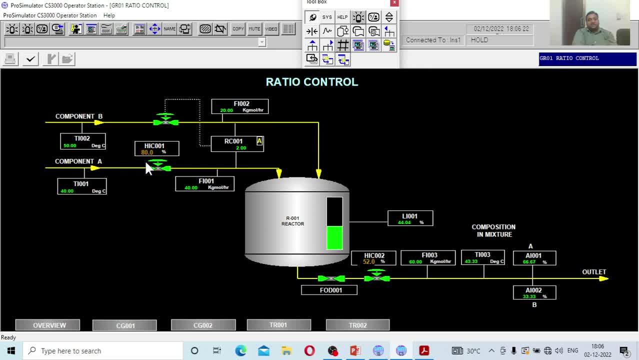 What happens? let us say there is some disturbance that went into this particular tank. ok, imagine that now it is 80 percent open. what I am going to do is, if I reduce, I mean because the there is some problem with the this particular stream line. So suddenly I mean the flow rate of A has been reduced. ok, see accordingly the ratio. 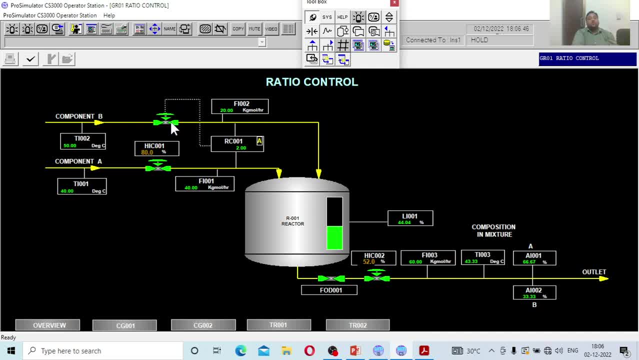 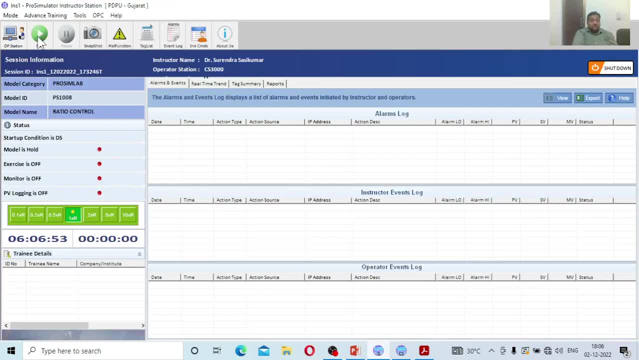 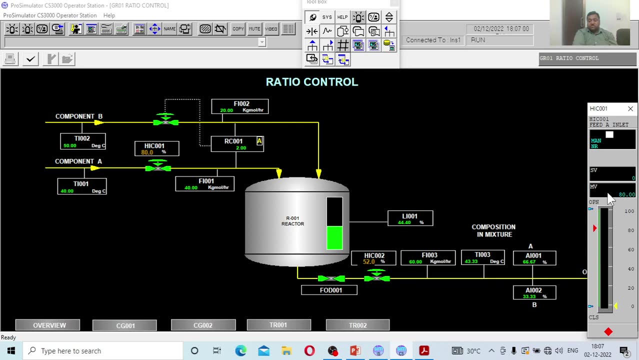 control will take action. it will also reduce the amount of B to that of A according to this ratio factor. ok, Let me, let me start this training program and this, let me HIC controls. let me close this, well, a bit. let us see what happens. ok, I am going to close this. well, what you people 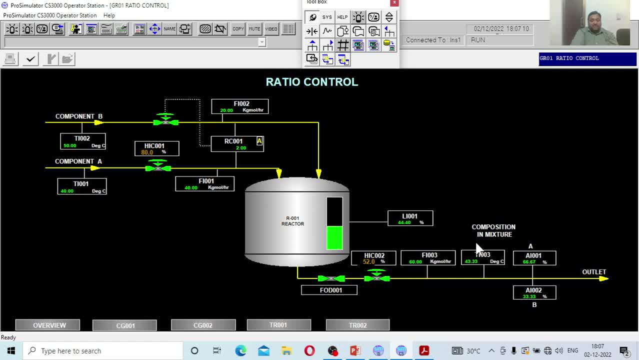 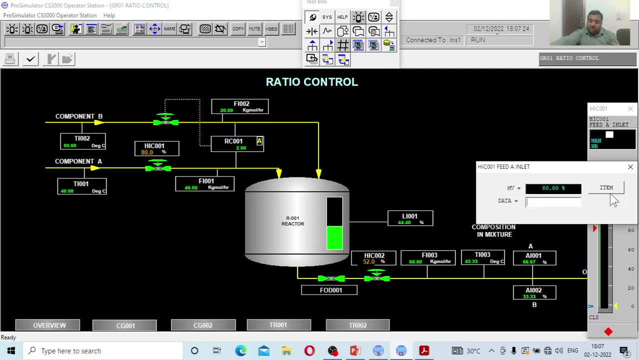 have to observe simple, whether is it maintaining the same percentage or not, exactly whether, if I reduce the A, is it stoichiometrically the amount of B also getting reduced through the ratio controller? So you need to check. ok, let me reduce to 60 percent. ok, and see each and every parameter. 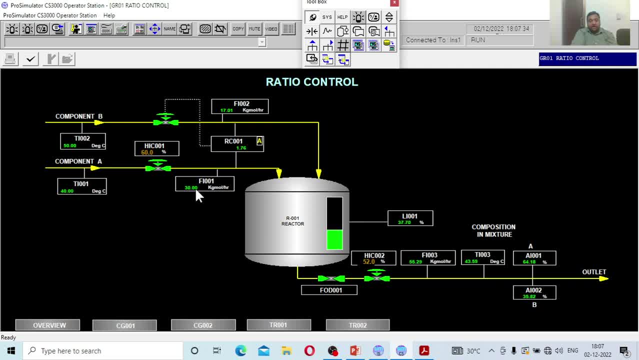 the flow rate of A has been now reduced to 30. now accordingly, it should be 15, but B should be 15, because the ratio control, I mean now the ratio, has been disturbed here. what is the set point is 2, what is the process value is 1.95.. 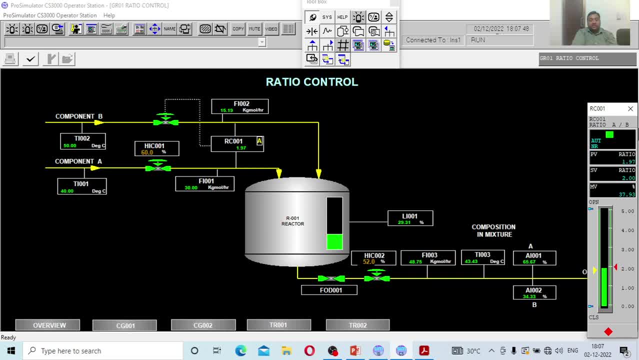 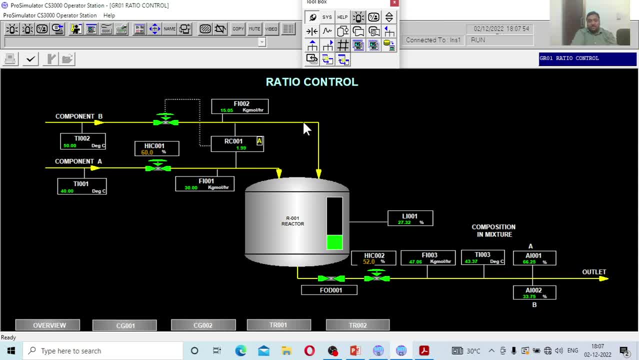 So now it is got disturbed. So now it is got disturbed. B, also to the stoichiometric amount, which is 15. ok, let me check. see the dynamics. it is a very simple. it is a kind of feed forward. see why it is feed forward before it is the 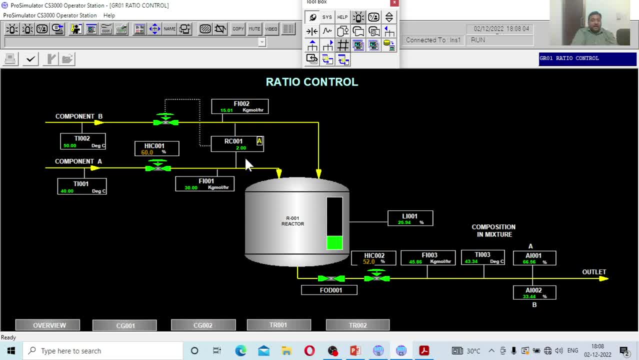 reactor getting disturbed, and early it. it is taking action before the A is getting entered into the reactor, So immediately it will. it will sense the change in the flow of A according to the ratio controller will take action immediately. it will close the valve to maintain the ratio. 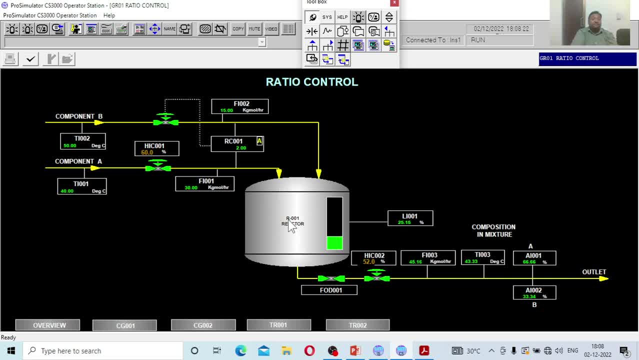 before it enters the reactor. that is why it is called feed forward. ratio control is one such of a controller. it is called a feed forward controller. okay, you can do many things here. right now i have i did the servo problem. now i mean, i did the- i mean disturbance problem. 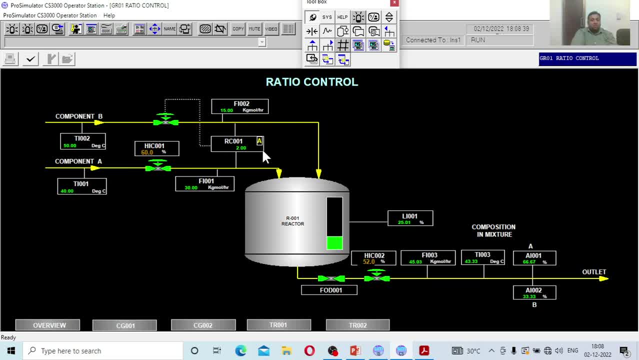 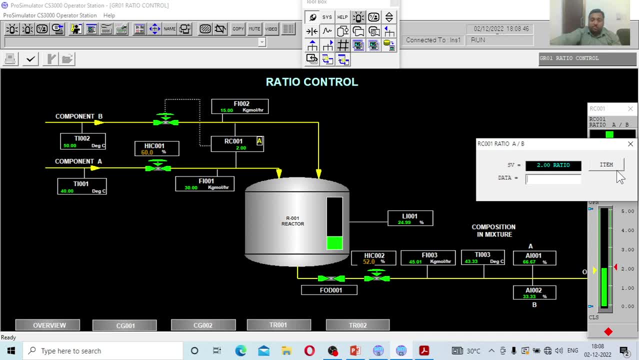 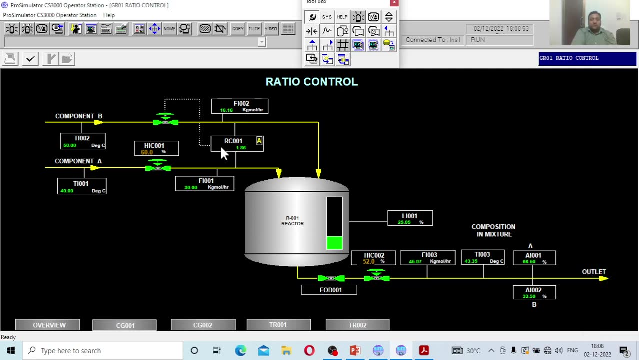 now i do the servo problem. see, everything got restarted. now i want to change the set point because my strike. i wanted to change my stoichiometric. what i do, i simply set point is 2, now it make it 1. okay, i want to send equal proportions of b in a. now see i ratio. 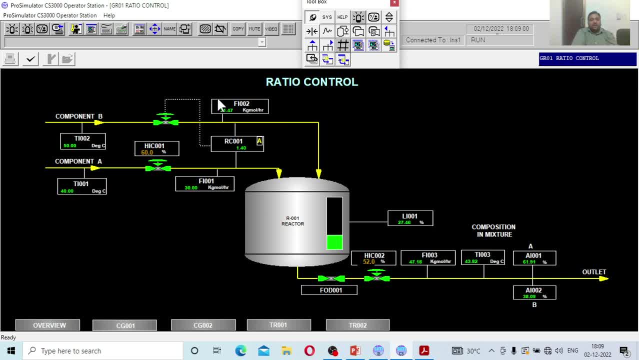 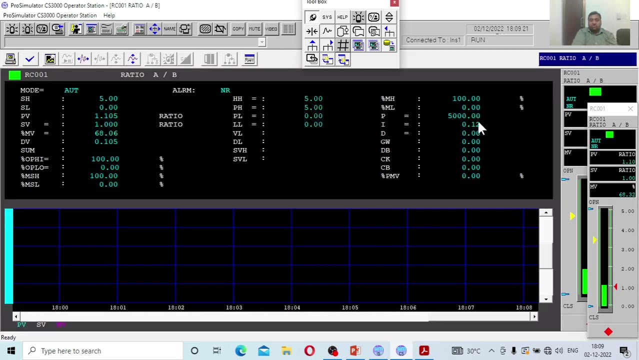 is, i mean 1. now a is 30, b is also should reach to 30 because i have changed my set points here. okay, in this i can apply many factors. let us say, if i go right, okay, let me check, i can turn it to the tuning. i can do tuning also. right now it is i controller. 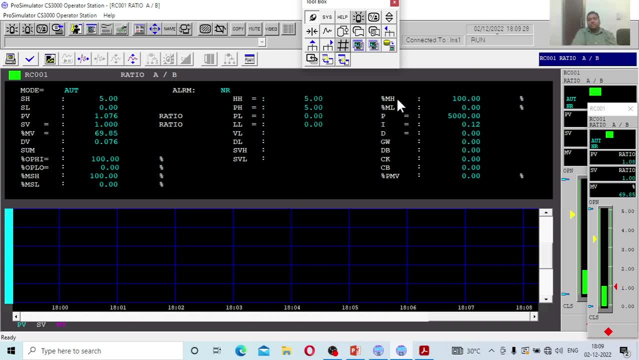 only integral controller and you can do many variations in the simulator. that means you can able to bring in pro- i mean pid id also, derivative control also, and see how fast it is going. it is almost getting reacted instantaneously. but if you bring in some derivative action, 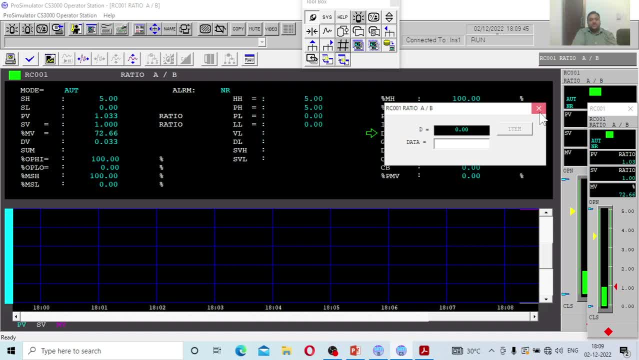 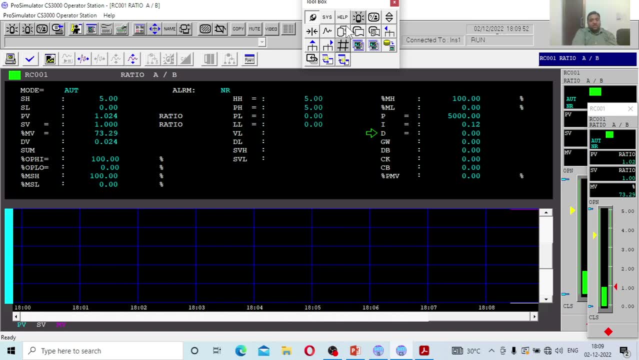 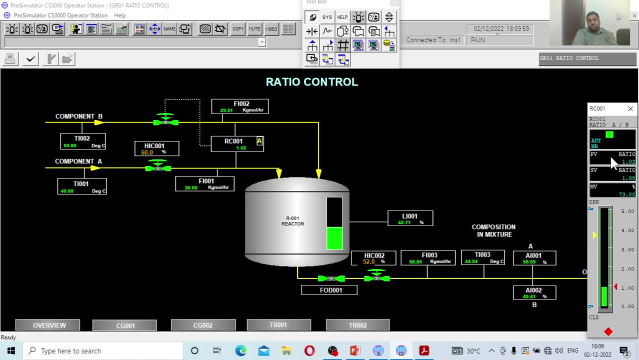 here by putting some number, so automatically you will see the number of the action and see what, how p controller and how pi controller, how pid controller is getting reacted to the different situations. okay, this is how, and now see the ratio. it is getting close to the set point. what is the set point? this is 1 and process value is of the 1.02. still it. 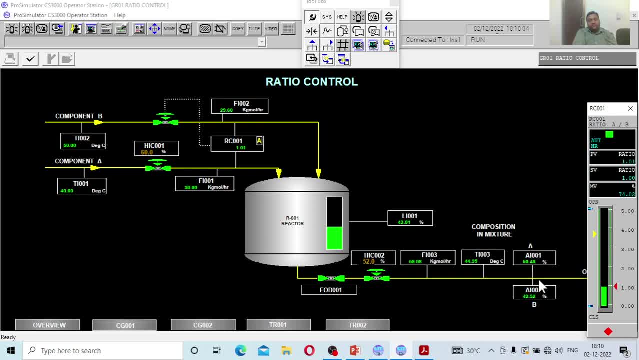 is going to take one more action and they see the exit composition now: 50, 50, 49.52 of b and 50.44 of a, because equal amount of kg mole per hour of a and b are going inside. so ultimately the composition will be 50 percent a and 50 percent b. if you want to see the 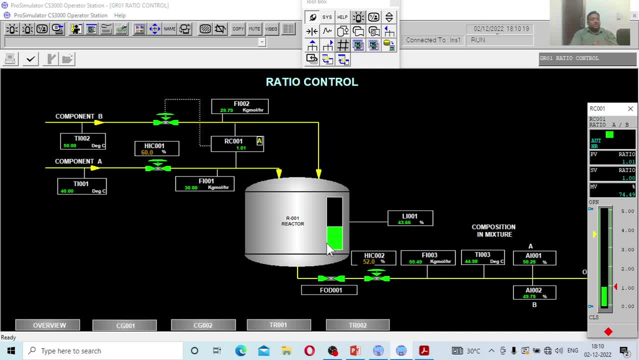 inside this time. so this is what the simple ratio controller and i have explained hope now. now you should be okay with the all the different controls because in the next phase we are going to do a bit advanced kind of no processes, let us say operation of a discussion. 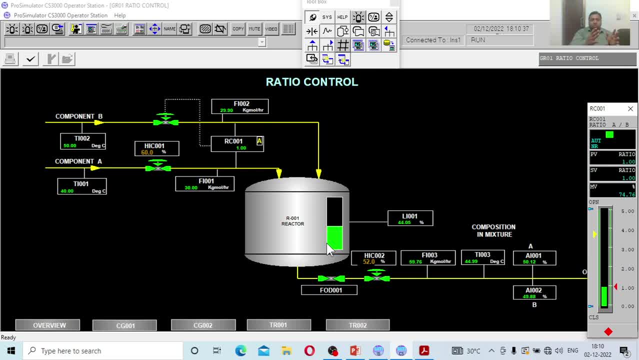 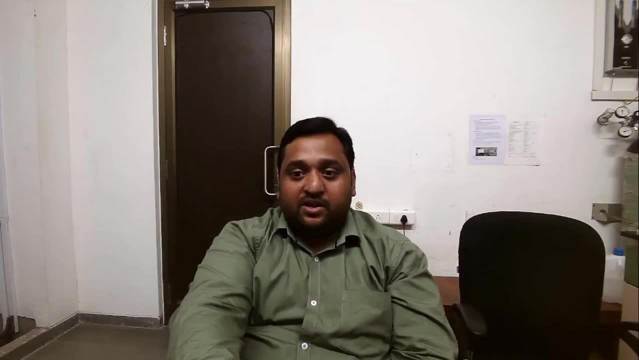 column operation of a csts. as long as you do not know this basic, you know, like example, ratio control, feed forward, feedback word, what is split range control, what is capitalized cascade control. if you let me come to the video, then i will put more amount of yeah. 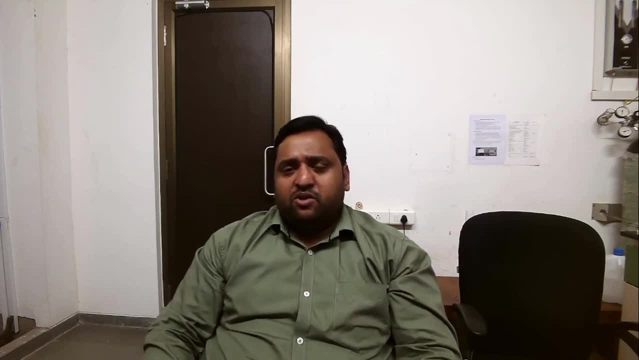 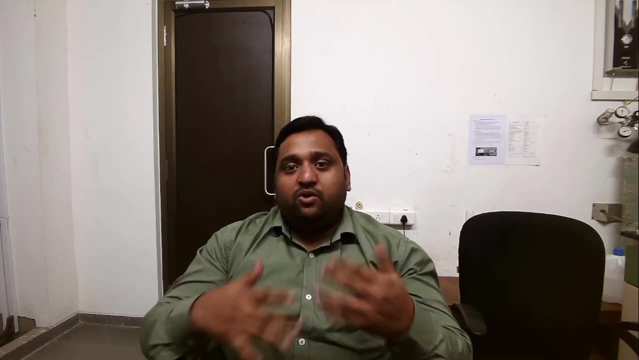 and we have uploaded almost close to, i mean, 12 kind of videos and before we jump into the next level of controls, of course i will take some time to upload those videos. i want you people to be acquainted with the- i mean present and different modules we have covered. 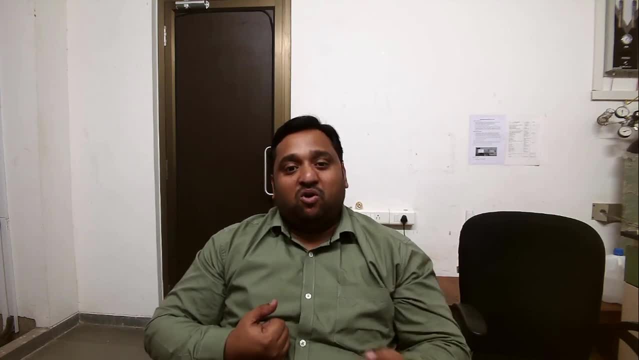 like feed forward control, feedback work control, what is on off control, what is split range control, care control, what is a direct control? and- and today we have discussed something about the ratio control. if you are okay with the, all the controllers know, and then you easy for you to understand the. 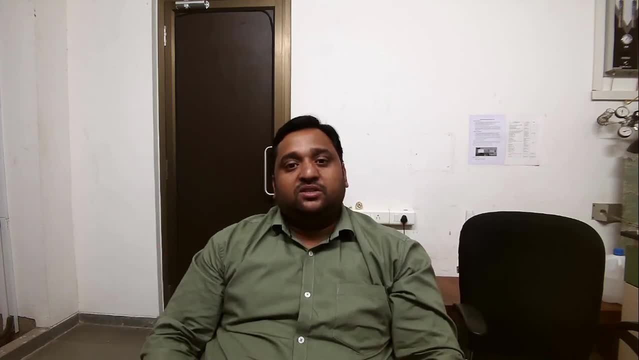 next phase. okay, those who could not able to watch the present videos, i strongly it's a mandatory for you people to go to the all the other video, previous videos, to get an idea of overall objective. so i hope you are. i mean, what is the objective of this particular process? you people? 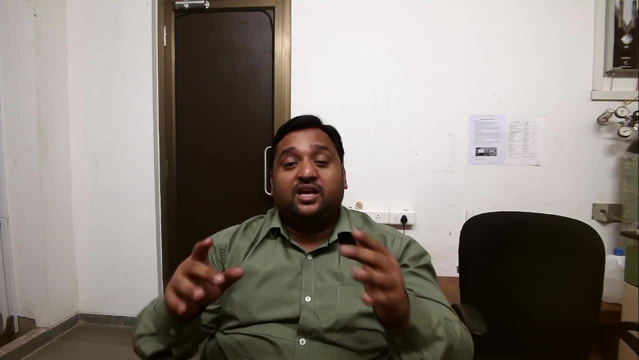 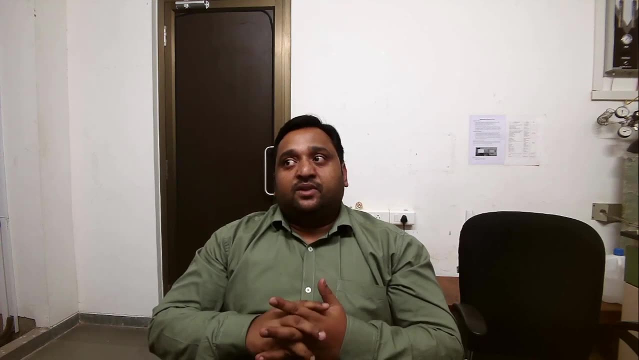 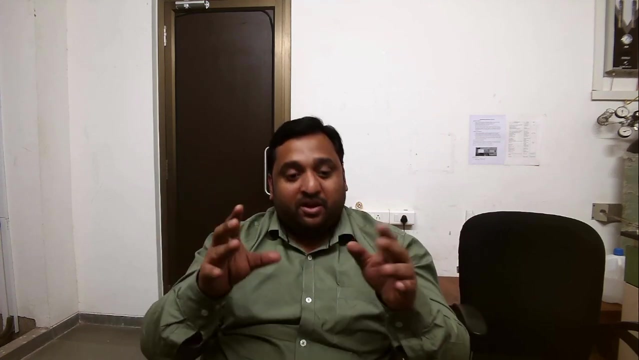 to get acquainted what a chemical engineer does as an operator in an industry, if you get somehow know about this. basic processes and the screen. what is there on the screen? how, what are the controllers, how i can table to action, how i have to change the automatic mode to manual mode. you